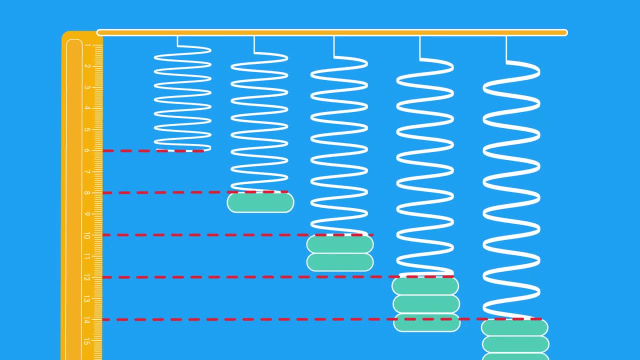 The extension of a spring is found by subtracting the original length of the spring from its length with the force applied. 2 N force extends the spring by 2 cm. 4 N by 4 cm up to 8 N and 8 cm. Hooke's law states the extension. 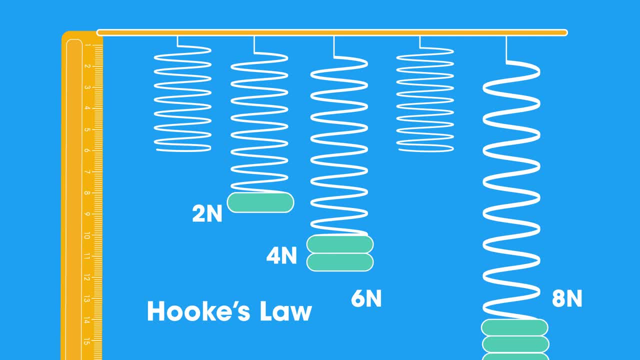 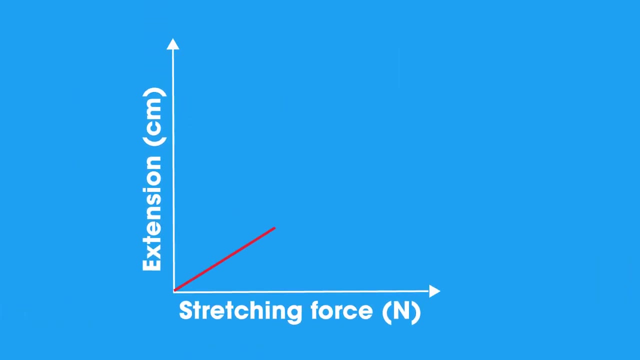 is directly proportional to the force applied, provided that the elastic limit is not exceeded. At the elastic limit, the spring becomes overstretched and won't return to its original state. So, to recap, the straight line shows that the extension is directly proportional to. 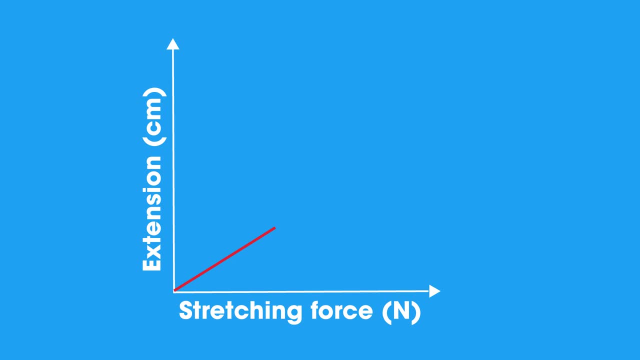 the load on the spring. That means the extension will double if the force doubles. it will treble if the force trebles, and so on. This relationship is known as Hooke's law. There is a linear relationship between force and extension. Here's the graph we get if we 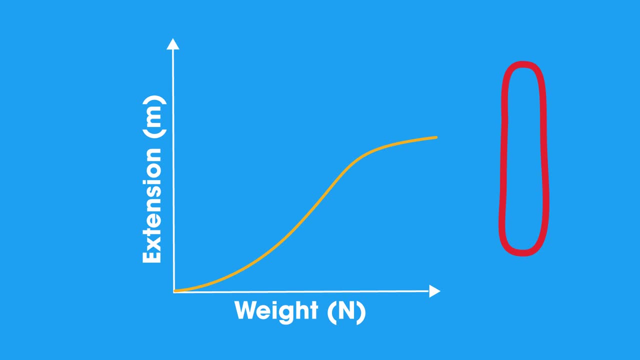 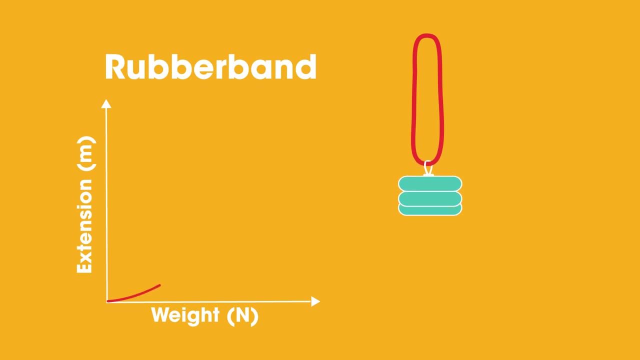 perform the same experiment, but use a rubber band. The result with a rubber band does not give a straight line graph, As weights are hung on a rubber band. to start with there is hardly any stretching. Then it stretches a lot before almost stopping as the band is extended fully. This is an example of a non-linear relationship. 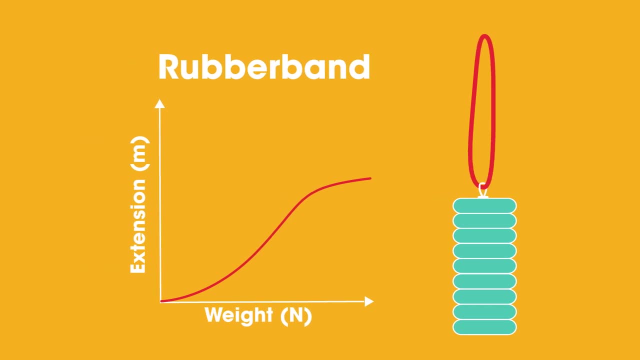 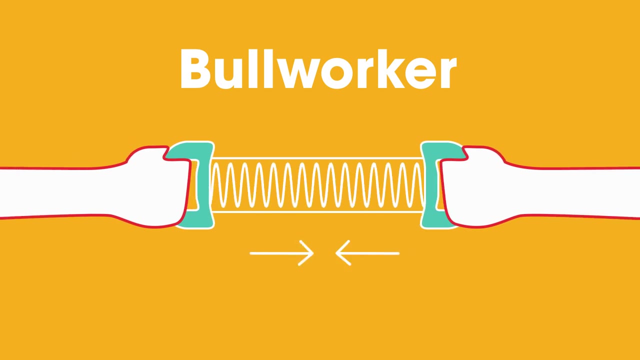 and the band doesn't obey Hooke's law. This machine, called a bulwarker, is used to exercise muscles. When the ends are pushed inwards, the spring inside is compressed. The bigger the force, the more the spring is compressed If the force is gradually reduced. 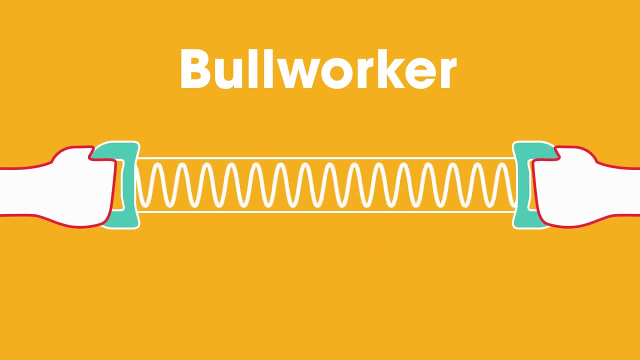 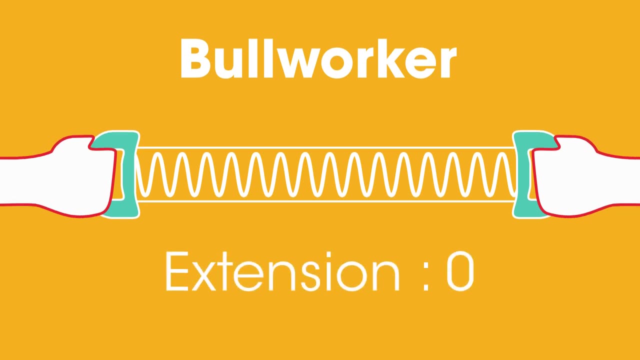 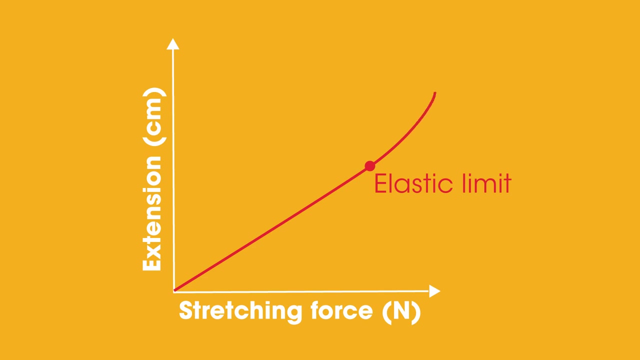 the spring expands until it regains its original shape. The spring is showing that it has elastic properties. The extension returns to zero. We can see this at the origin on the graph for the spring experiment. This spring obeys Hooke's law When the weight and the upward or restoring force are 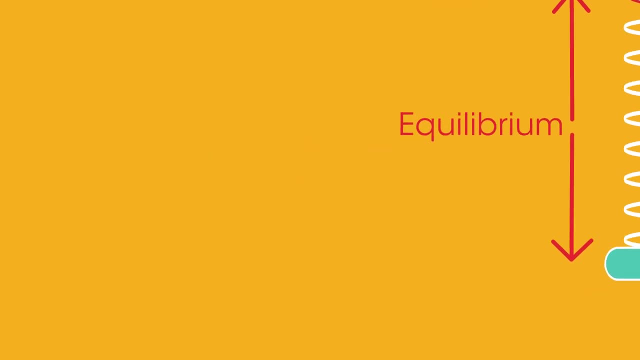 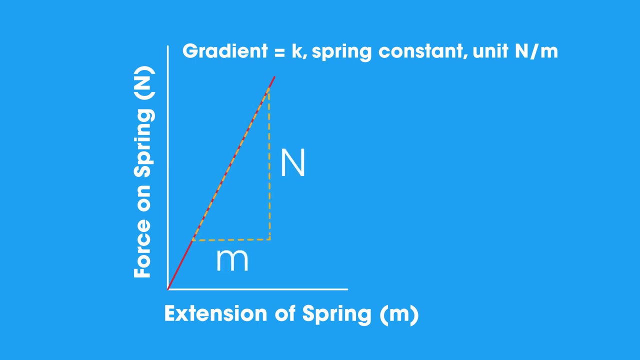 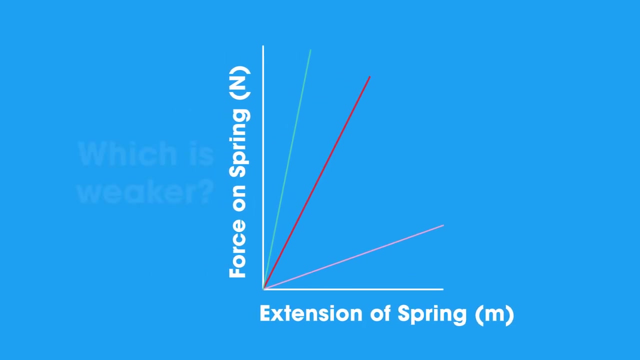 equal, the spring is said to be in equilibrium. The spring constant K is a measure of the strength of the spring. It measures the force or the number of newtons it takes to stretch the spring by one metre. Which is the weakest spring- A, B or C? 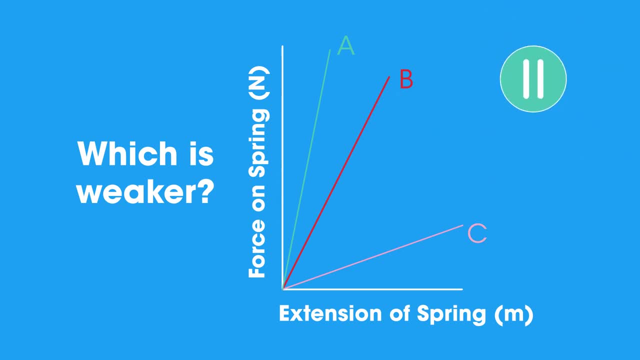 Pause the video and check out our other videos. Thank you for watching Well, C is the weakest spring, needing only a small force to make a big extension. And which spring will store the most energy if they are all extended by the same amount? 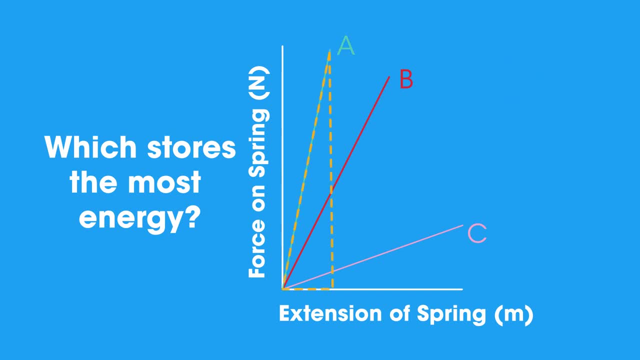 Spring A will store the most energy because it needed the largest force. Let's look more at the stored energy. When we stretch a spring, we can see that the energy stored in the spring is the largest force. When we stretch a spring, we can see that the energy stored in the spring is the 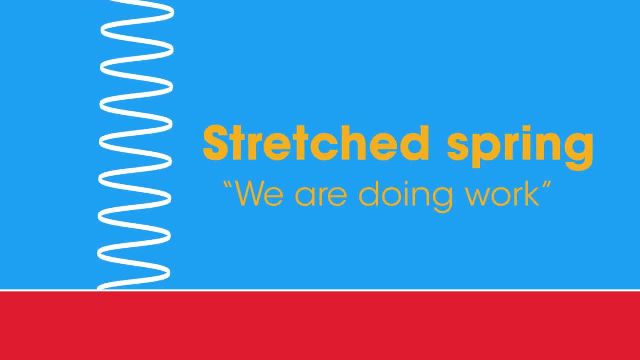 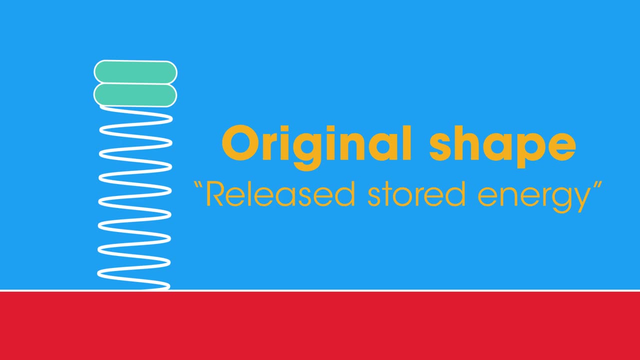 largest force. When we break a spring, we can change its shape Anytime the saràc is stretched and we are doing work. When we do that, We can avoid another spiral with a product to create newtsons. The spring can then go back to its original shape and the energy stored in it is released. 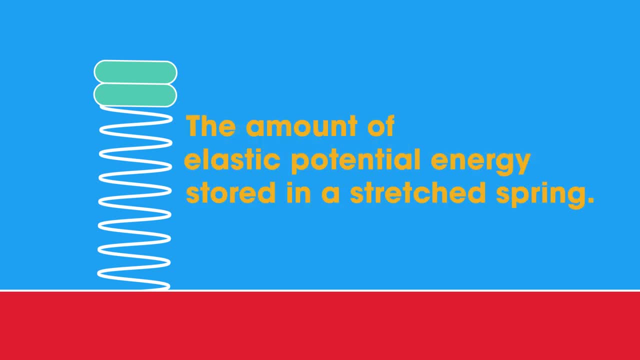 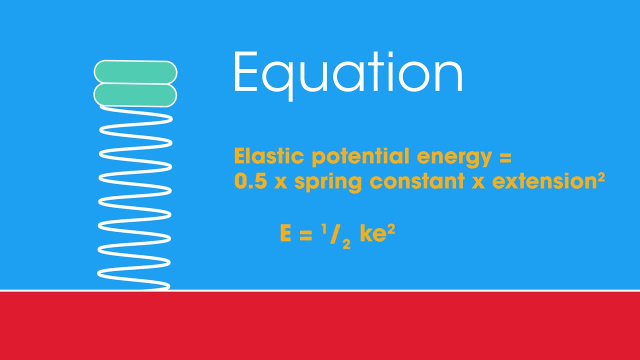 The amount of elastic potential energy stored in a stretched spring can be calculated using this equation: Elastic potential energy equals to 0- .5 times spring constant, times extra strength squared, Asuming the spring obeys Hooke's law where elastic potential energy E is measured in Joules spring constant K in. 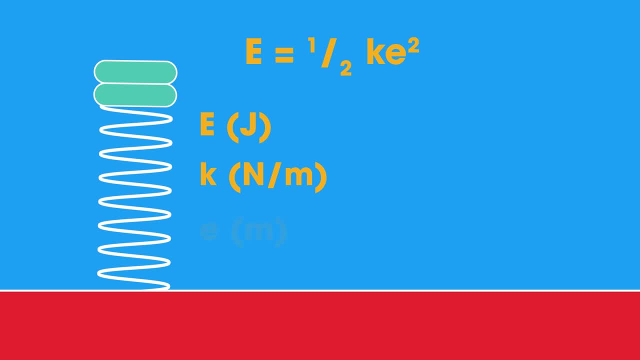 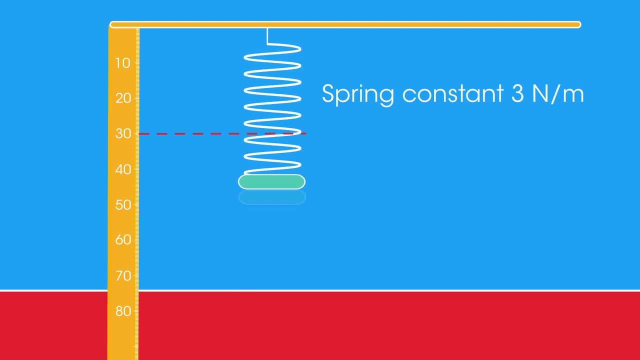 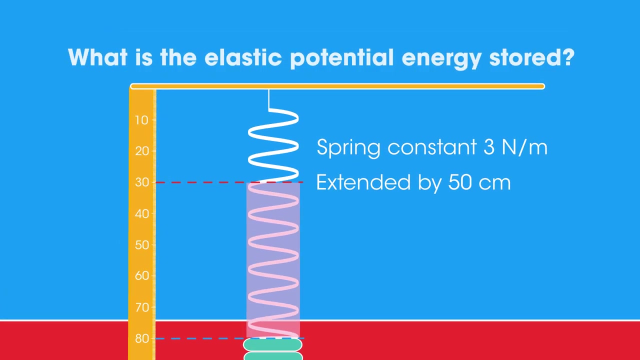 Newtons per meter and extension E in meters. Let's try applying this. A spring is stretched. It has a spring constant of 3 Newtons per meter. It's extended by 50 centimeters. What is the elastic potential energy stored by the spring? 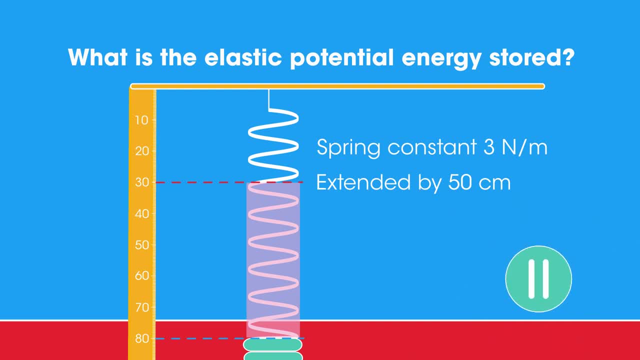 Pause the video while you work it out. How did you do So? that's everything you need to know about the springs and their extension. 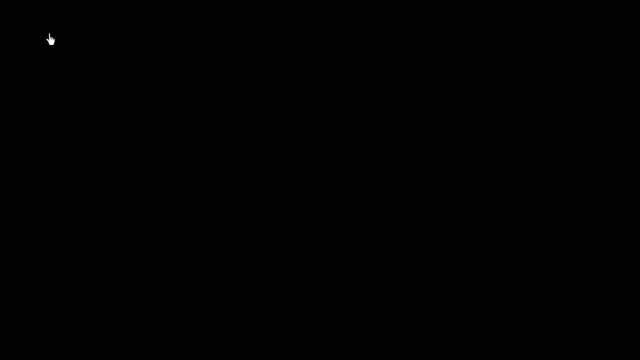 Let's have some practice adding and subtracting negative numbers. So the first example I want to look at is 2 minus 3.. So right now I'm just subtracting a positive number from another positive number, but you might already see that I'm subtracting a larger number.